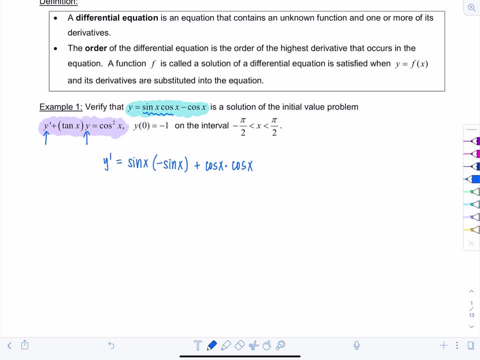 and then leave the other cosine x alone, And then derivative of negative cosine x is going to be positive sine x. So all we're left with here now is negative sine squared x plus cosine squared x plus sine x. So that's y prime. 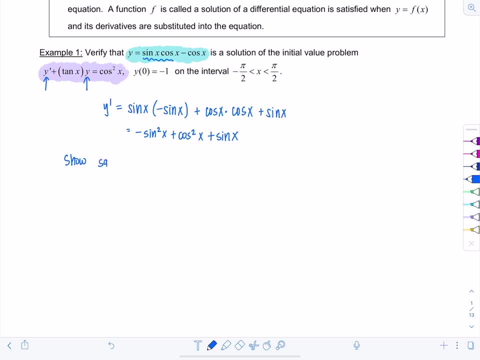 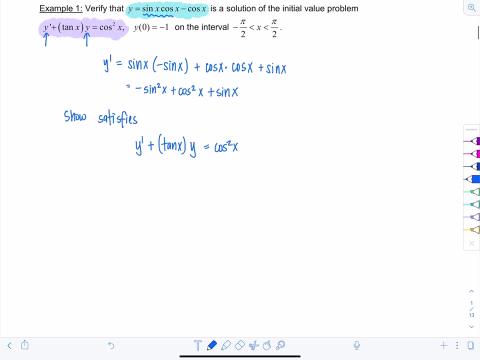 Now I want to show that it satisfies the equation that was given. y prime plus tangent of x times y equals cosine squared x. So to begin, I'm going to substitute in for y prime the derivative that we just got right here, So negative sine squared x plus cosine squared x plus sine x. 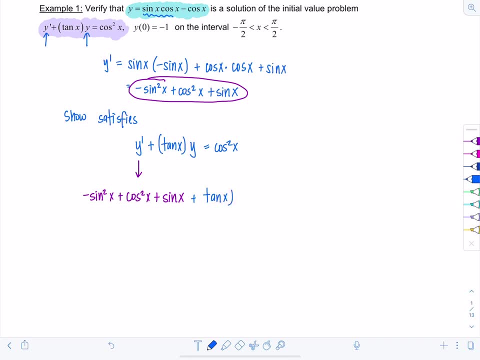 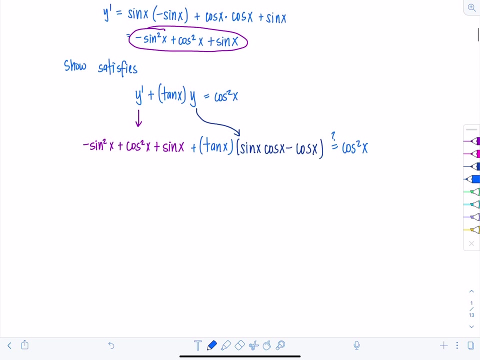 And then I have plus tangent of x times. now I need y, the original function, which is right here. That was my original y. So sine x, cosine x minus cosine x. And I want to confirm: does this indeed equal cosine squared x? Let us see. So we have here negative sine squared x. 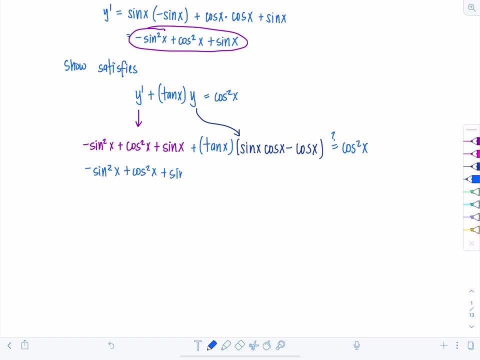 plus cosine squared x plus sine x. Let's distribute this: tan x, Okay, and I know tangent x is sine x over cosine x, So it's going to cancel with that cosine x here and I'm going to be left with plus sine x. 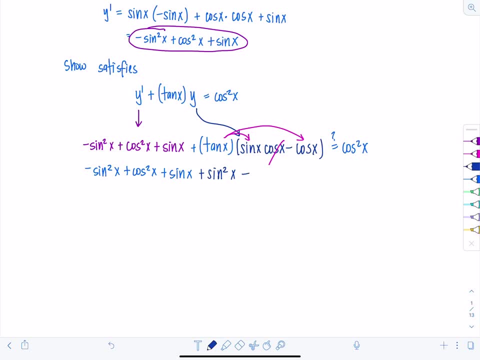 So sine squared x minus, and then it's just going to cancel with that cosine x over there and I'm going to be left with sine x. So does this equal cosine squared x? I see quite a few terms I can cancel, don't you? So sine squared x is gone, Bye-bye. 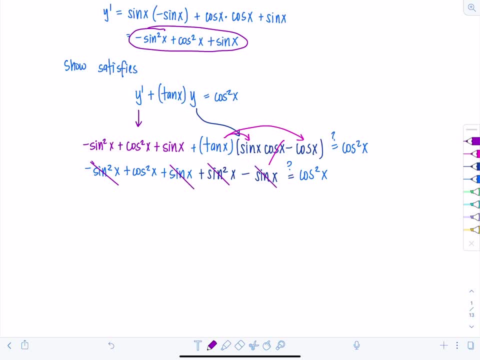 Sine x is also gone. So yes, cosine squared x equals cosine squared x. So we've verified that that particular equation is a solution for the differential equation that was given. All right, very good, Let's look at some other kinds of differential equations. 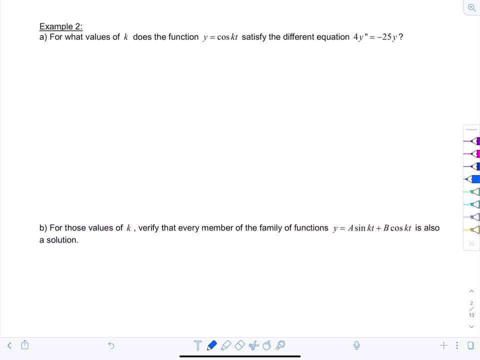 Example two. So for what values of k does the function y equals cosine of kt satisfy? the differential equation for y, double prime equals negative 25? Y. So this differential equation that we're working with is different than the previous one because- notice it's second order, We have a second derivative in it And what we're going to do is: 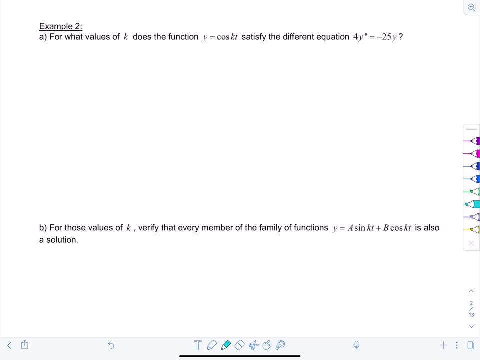 find k, the constant in particular that we need in order to satisfy this differential equation. Okay, well, we're working with the function y equals cosine kt. That means y prime would be negative using the chain rule Y sine kt. So y double prime. I'd multiply by k one more time and have negative k squared. 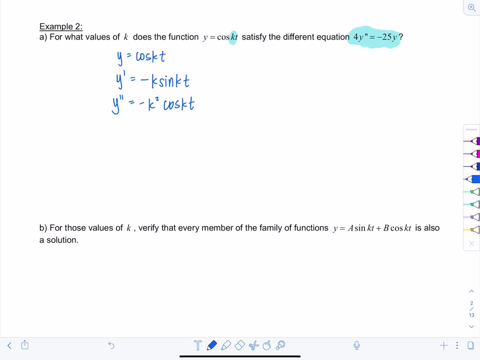 cosine kt. Okay, so now I'm going to substitute all of this into the differential equation that was given right. 4y double prime equals negative 25y. So 4 times y double prime is right here, negative 25y. 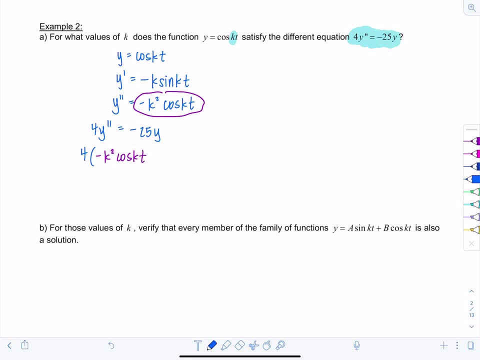 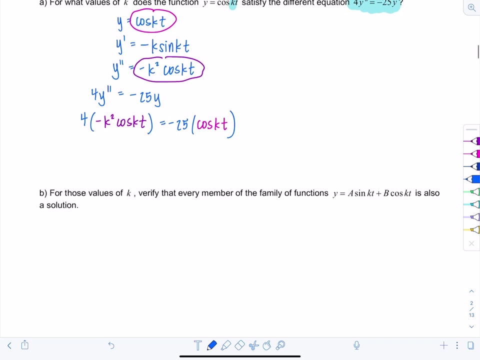 k squared cosine kt. That needs to equal negative 25 times y, the original, which is right here- cosine kt. Okay, so to solve this equation, let's set it equal to zero. So I have negative 4k squared cosine kt plus 25 cosine kt is zero. 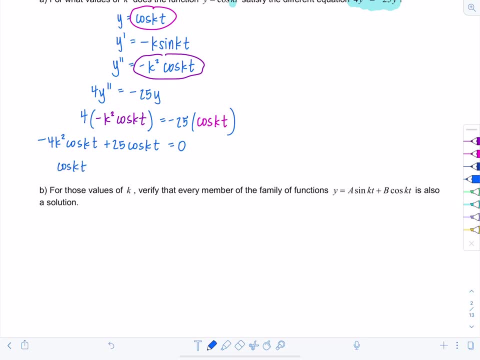 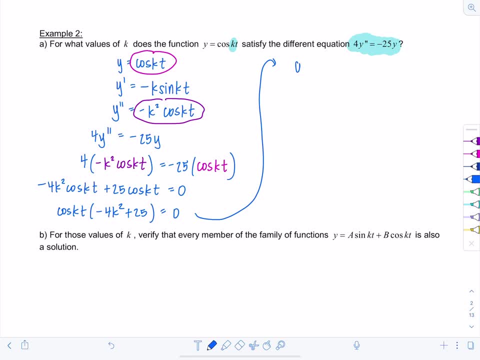 property. now to solve: Either I get cosine of kt equals zero or negative. 4k squared plus 25 is zero. Now, if cosine of kt equals zero, that's just the trivial solution. What do we mean by that? well, they're telling me, the equation has the form: y equals cosine kt. So obviously, if y is, 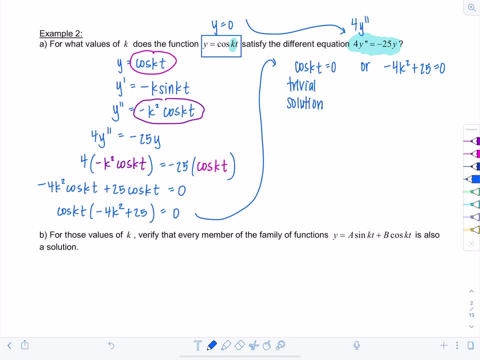 equal to zero, then four times y, double prime would be four times zero and that would equal negative 25 times zero. If your function is just zero and you keep differentiating, you're going to get zero and it's going to satisfy it. That's why we say it's a trivial. 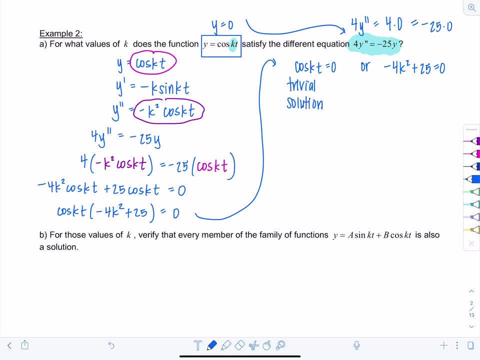 solution. It's not interesting, It's obvious case: Function is constant. Now this one. here we go. We're going to get something interesting happening. k squared would equal 25 over four, which means for k we get either plus or minus five halves. Okay, very good. 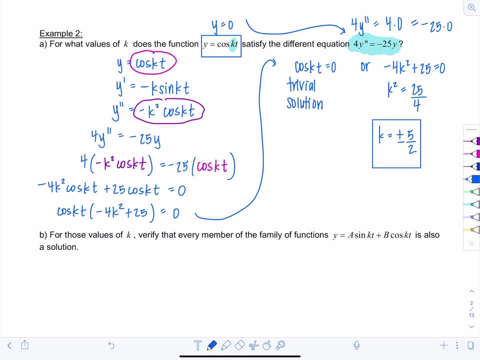 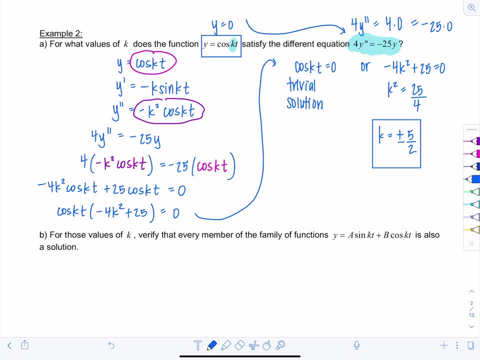 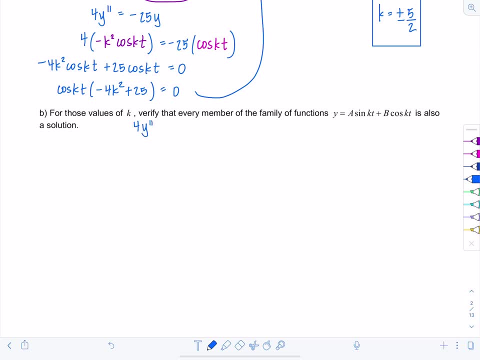 original differential equation which says that 4y double prime has to equal negative 25y. So if this is what y is equal to, let's see what y double prime would be and then verify that it's going to satisfy it. So y prime I'm going to differentiate now. So derivative of a sine kt. 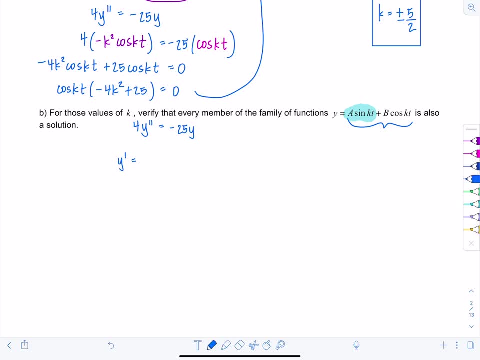 I'm going to have to multiply by k right, because of the chain rule. So I'm going to have k times a cosine kt and then derivative of the next term is going to be negative: k times b sine kt. Okay, one more round. Remember we need y double prime for this equation. So now this is going to: 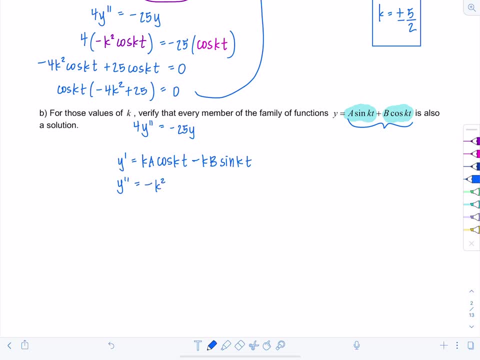 be another chain rule. another k is going to get multiplied out, so negative k squared a sine kt. So I'm going to have k times a cosine kt and then derivative of the next term is going to be negative k times b sine kt and this is going to stay negative minus k squared b cosine kt. 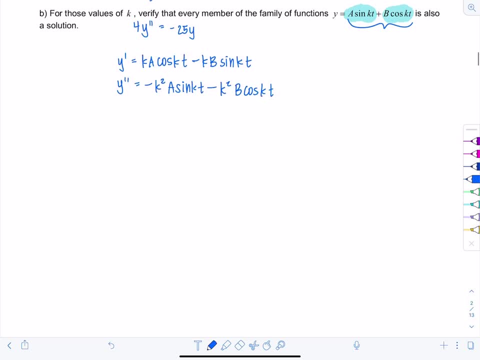 Okay. so now let's check if this satisfies the differential equation. So 4 times here's y double prime. let's plug it in here. negative k squared a sine kt minus k squared b cosine kt, Does that equal negative 25 times y, y being the original guy right Here, a sine kt plus b cosine kt. 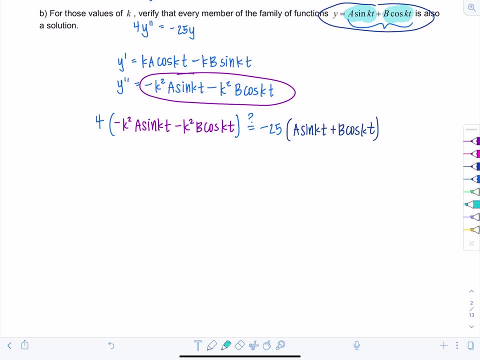 Okay, let's see what we can do to clean up. Oh, I can factor out a negative k squared, Do you see that? Okay, so we've got negative 4k squared. So we've got negative 4k squared, and then we've got. 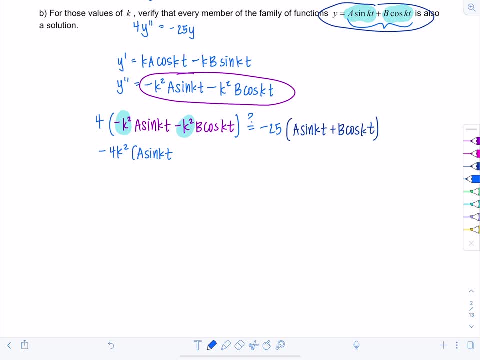 negative 4k squared times a sine kt plus b cosine kt. And I want to know: does that equal negative 25 times a sine kt plus b cosine kt? Well, what did we get for k? Remember we got for k previously that it was equal to plus or minus 5 halves, which means that k 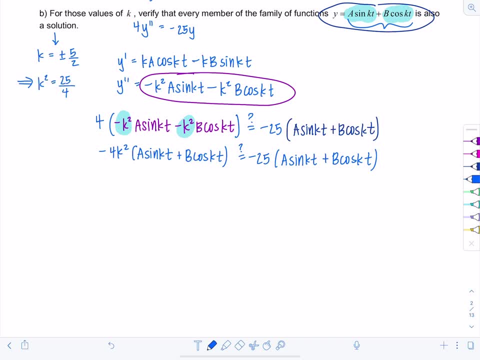 squared was equal to positive 25 over 4.. So if I substitute that in for the k squared here on the left, I'd have negative 4 times 25 over 4 times a sine kt plus b cosine kt And I can see yep. 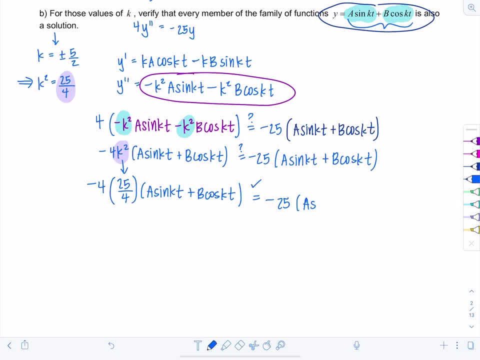 that equals negative 25 times a sine kt plus b cosine kt. Right, depending on if you choose the positive or negative, these will cancel out and you get the same thing on both sides. So it's verified. Make sure until you verify at the final step. 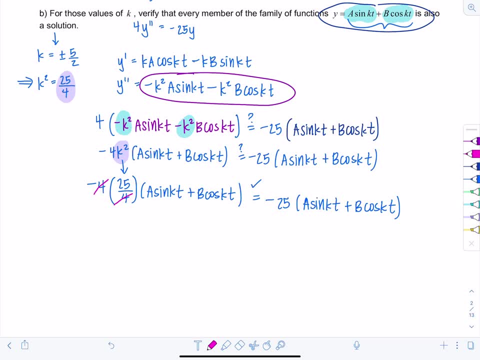 you're putting that question mark above the equal sign. You don't want to write it like: oh it's already true until you've actually verified it right. Okay, one more example: Show that every member of the family of functions. 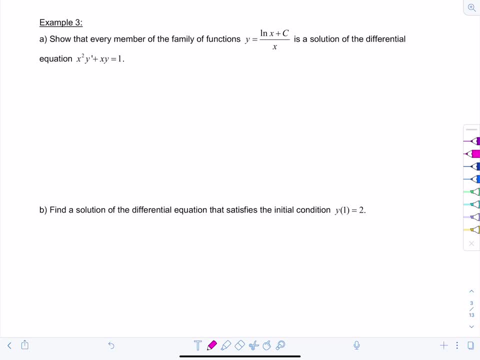 y equals natural log of x plus c divided by x is a solution of the differential equation. x squared y prime plus x times y equals 1.. Okay, so this is a first order differential equation. I just have first derivative in there, So let's go ahead and 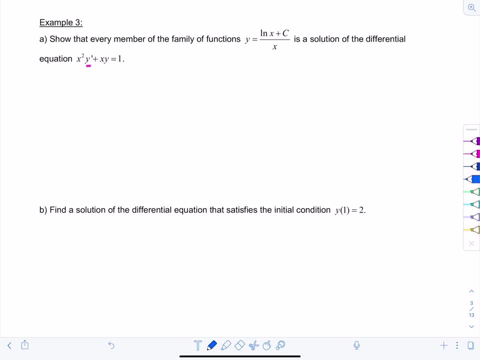 compute it, plug everything back in and verify. So y prime, we've got to use the quotient, We've got to use the quotient rule. So we have low to denominator d, high, derivative of the top. That's 1 over x plus. see, it's just a constant. so 0, minus high d low over the denominator squared. 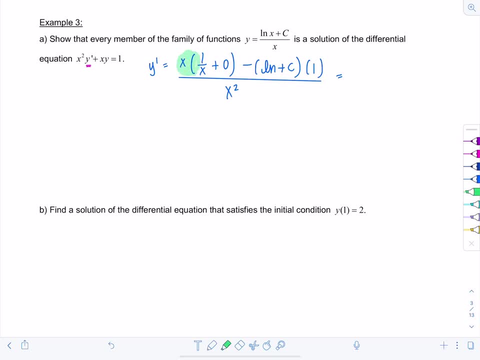 And then this is going to clean up: x times 1 over x. That's just going to give me 1.. And then distribute this negative here, so minus ln of x, minus c over x squared. So I'm going to substitute this in now. 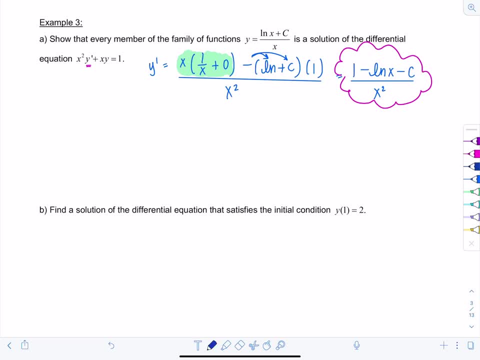 for y prime in the differential equation. So we've got x squared times 1 minus ln of x minus c over x squared plus xy. But for y, remember, I'm going to replace it with ln of x plus c over x And I want to see: does that equal 1?? Yeah well, this one's pretty easy, right? x squared. 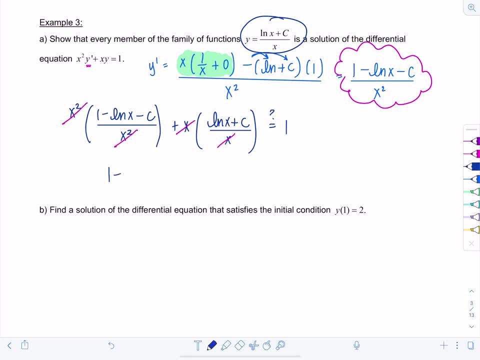 cancels x cancels. So I have 1 minus ln of x minus c, plus ln of x plus c. Cancel, cancel, cancel, cancel. Yep, that equals 1.. Okay, now notice, in this differential equation we had plus c, right, We had a more general solution. 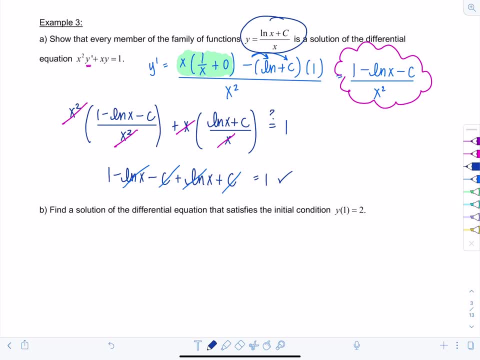 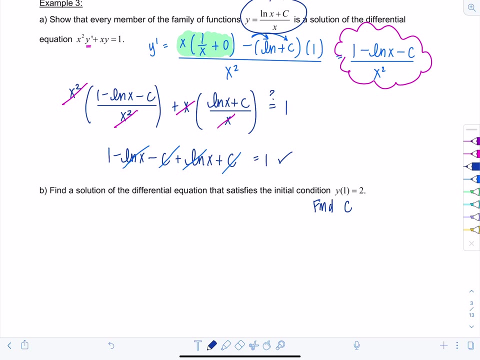 Here they want us to find a solution of the differential equation that satisfies the initial condition: y of 1 equals 2.. So, basically, what they want us to do now is find the particular c that yields the unique solution. So find c. That's what that's telling you to do. 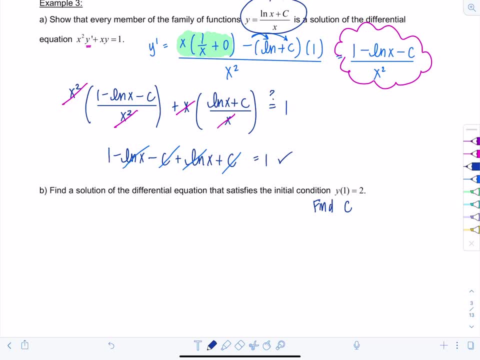 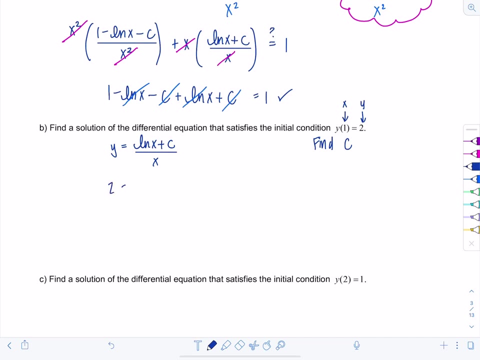 So you just have to go back to the family of functions that was given. as the solution. y equals ln of x plus c over x, And we're going to substitute in now 1 for x, 2 for y and solve for c. all right, So 2 equals natural log of 1 plus c over 1.. 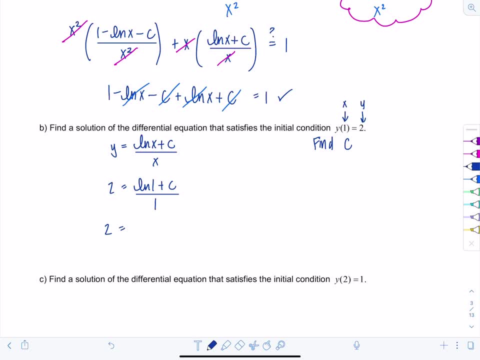 Well, that means 2 equals ln of 1 is 0.. So c equals 2.. So they want the actual solution. so put it back in. So y would equal natural log of x plus 2 over x. Okay, so when solving differential equations you'll see if you're not given an initial.